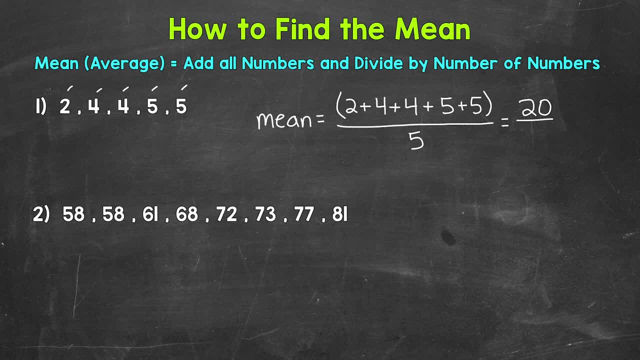 So the sum of the numbers is 20, and then we divide by 5.. So 20 divided by 5 is going to give us our mean. 20 divided by 5 is 4, so that's our mean for that data set. 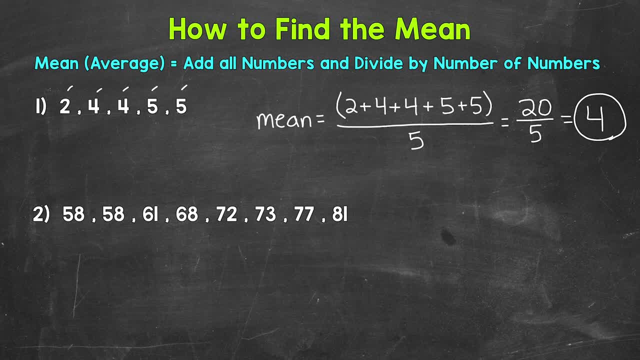 4 is one number or value that represents or describes that data set. So let's move on to number 2, where we have double digit numbers and then we have more numbers within our data set. Number 1, we had smaller numbers in value. 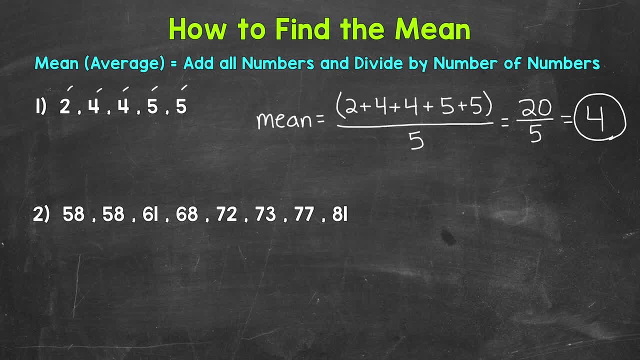 They were a little simpler to add. and then our mean worked out nicely, so to speak. We got a whole number. We had a 4 there. Let's see what happens with number 2.. So let's set this up: We have mean equals, and then we will add all of our numbers. 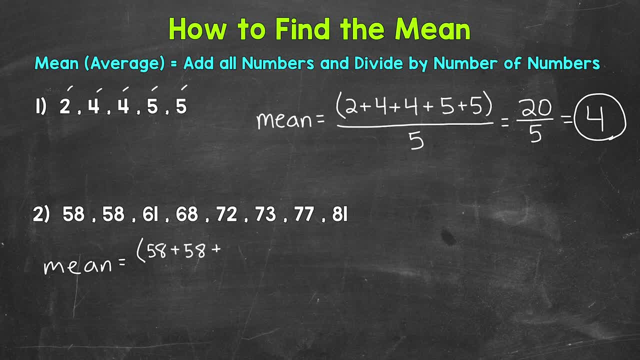 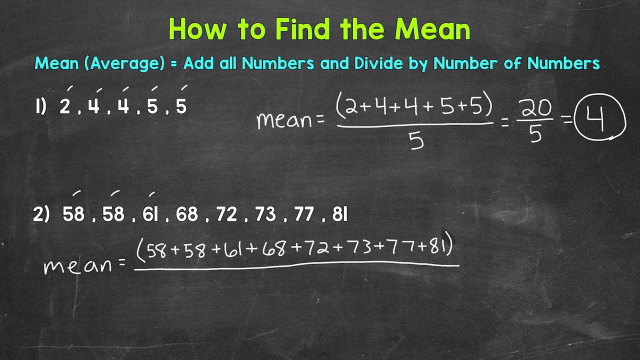 So we have 58 plus 58, plus 61, plus 68, plus 72.. Plus 73,, plus 77,, plus 81. And then we'll divide by the number of numbers in the data set. So we have 1,, 2,, 3,, 4,, 5,, 6,, 7, 8.. 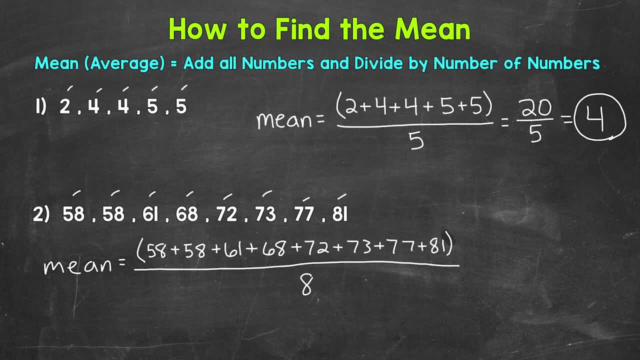 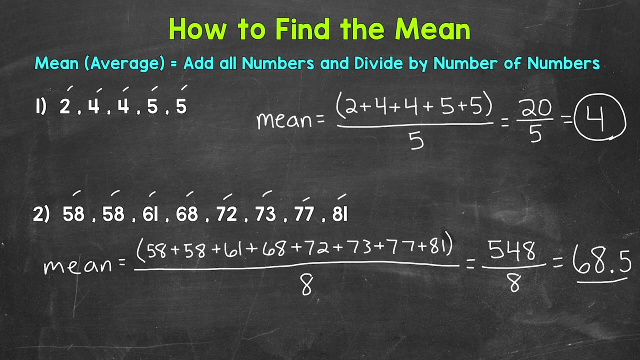 So we need to divide by 8.. Now we can calculate the sum of those numbers and it's going to be 548.. And then we divide by 8.. And then we divide by 8 to get our mean. 548 divided by 8 gives us a mean of 68 and 5 tenths. 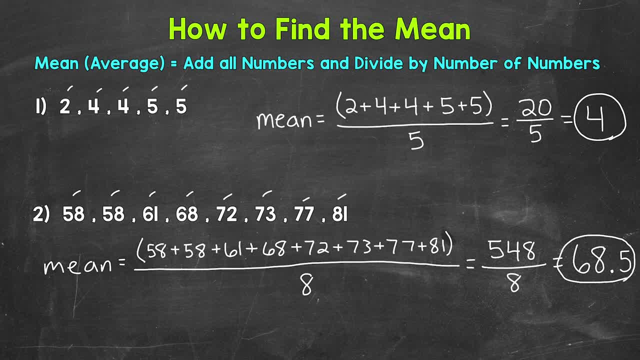 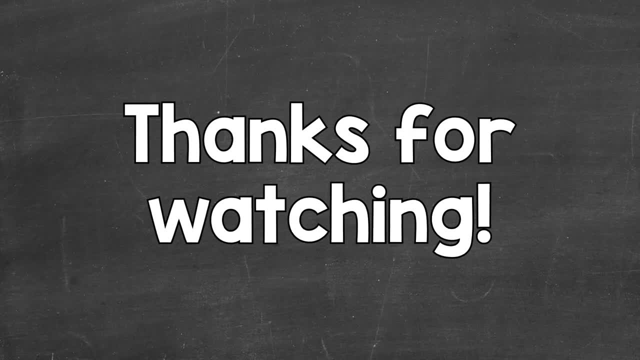 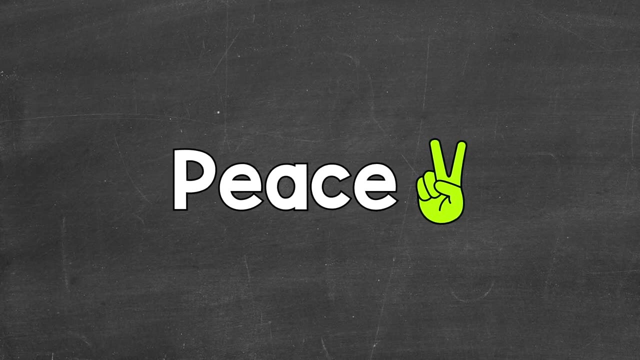 So 68 and a half is our mean for number 2.. So there you have it. There's how you find the mean of a data set. I hope that helped. Thanks so much for watching. Until next time, peace.